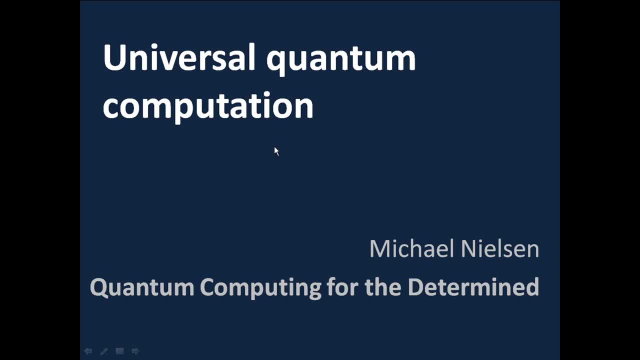 So we're now in position to put everything we've been learning together in order to understand the full model of quantum computation- what a quantum computer actually is. So let me remind you of a few facts that you already know about classical computers. We're 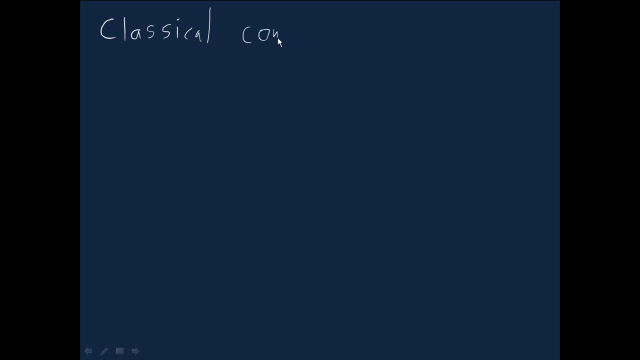 going to build on these facts in coming, describing the model of quantum computation. So the basic fact is this: So these conventional classical computers, as you know, you can take logic gates like the AND and the NOT gates and by composing them together you can compute any function. 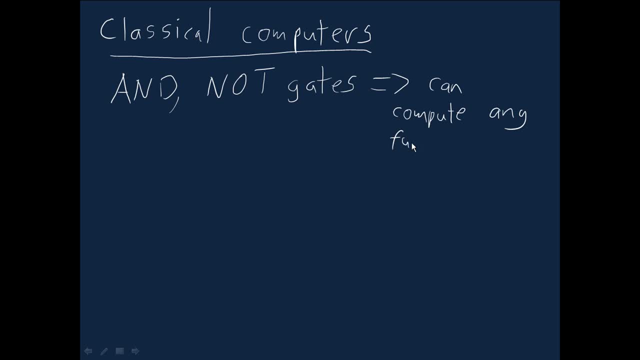 at all. In particular, this means that, without any loss of generality, you can build your computer, You can build your computing device up out of AND and NOT gates. So other gates, like the OR gate, or more complex things like addition, subtraction, multiplication, can be built up out of these basic 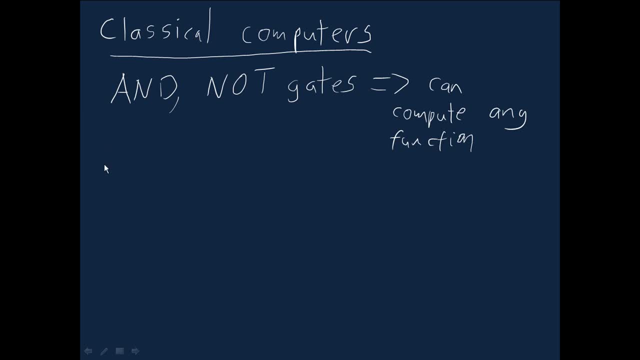 elementary operations. What we say is that the AND and NOT gates are universal for classical computation, And universal just means that you're able to use those to compute any function whatsoever. Of course there are other sets of gates which are also universal, For example the NAND gate. 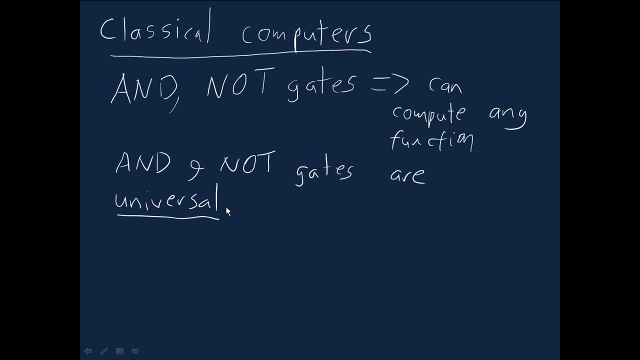 alone is sufficient to do universal classical computation, And there are many other sets as well, but they're all equivalent because, given one set, you can use that set to simulate another, And so the model of computing. you can use that set to simulate another, And so the model of computing. 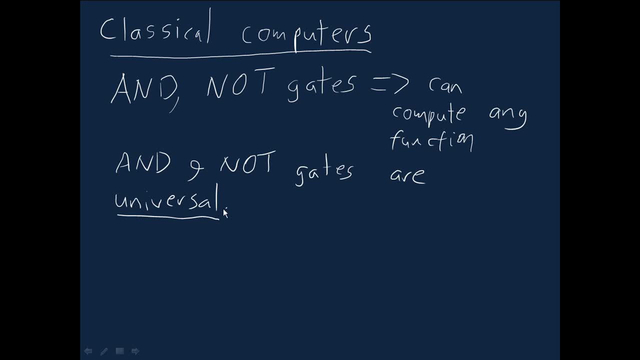 you get is essentially the same, because each model can simulate the other. Okay, so what's the analogous fact about universality for quantum computers? So what can we replace the AND and the NOT gates by in the case of quantum computation? And it turns out: 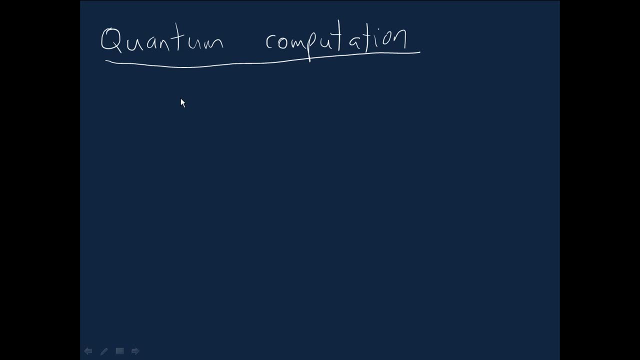 that in fact, the operations we've been looking at to date- the controlled NOT gate and the single qubit gates. single qubit unitary operations- can be used to build up any, in other words, an arbitrary unitary operation at all on n qubits. 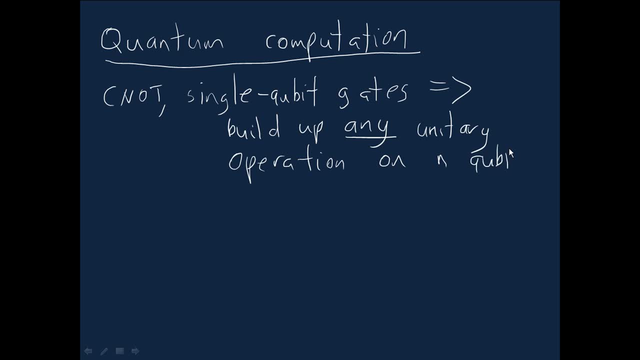 So n now is just some arbitrary number of qubits. In other words, if you pick any unitary operation at all on, say, 100 qubits, in principle it's possible to decompose into controlled- NOT gates- and single qubit gates. The proof of this fact I'm not actually going to explain. It's not terribly. 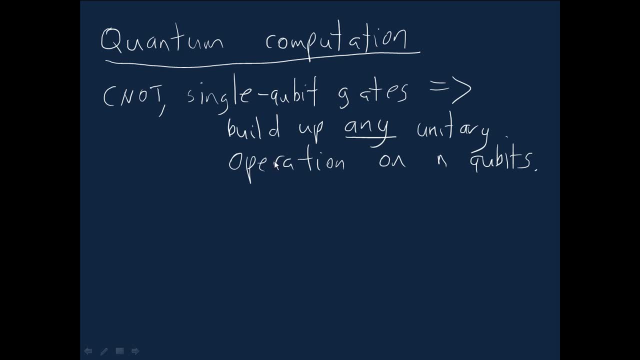 complicated, but there's quite a few details to go through, In fact, a lot of the sort of techniques that you need to prove this fact we will encounter later in the course. So you'll be well placed to understand the proof if you wish to, even though we're not actually going to do it. do the proof. 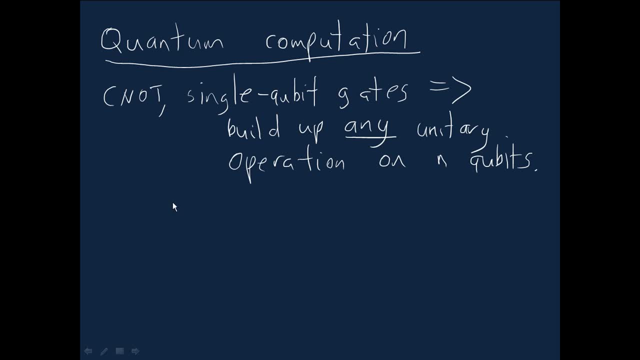 explicitly So we we say that the CNOT and single qubit gates are universal for quantum computation By analogy with the corresponding result for classical computation about AND and NOT gates. Now, of course, it probably won't surprise you to learn that many other gate sets are also. 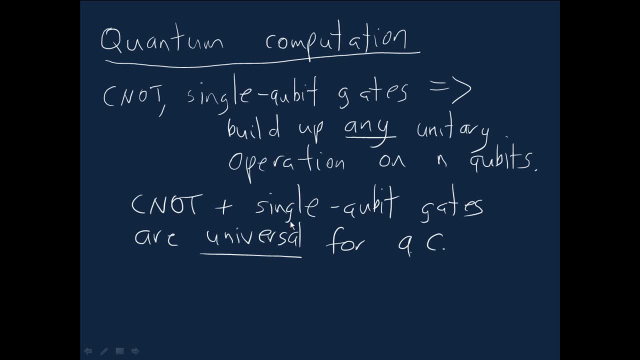 universal meaning that they can be used to simulate the CNOT plus the single qubit gates. So you know, it's not the only universal set, but it is one very convenient one and one that's very widely used. in practice it means that if you want to build a quantum computer, it's enough to be 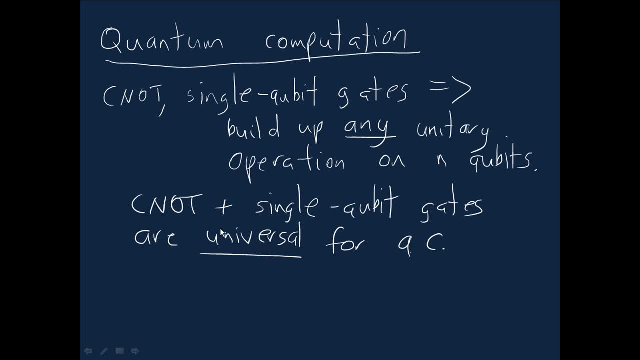 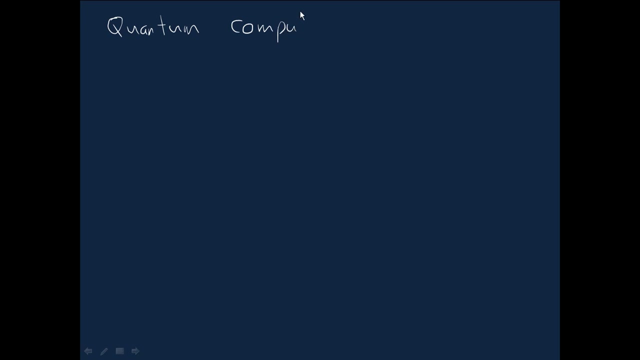 able to create qubits which are long lasting and also to do the c naught and single qubit gates plus measurements. okay, so let's actually be a little bit more precise about what exactly a quantum computation is. i'm going to explain it by example. i'm not going to write out a precise definition of a of a model, but you'll understand. 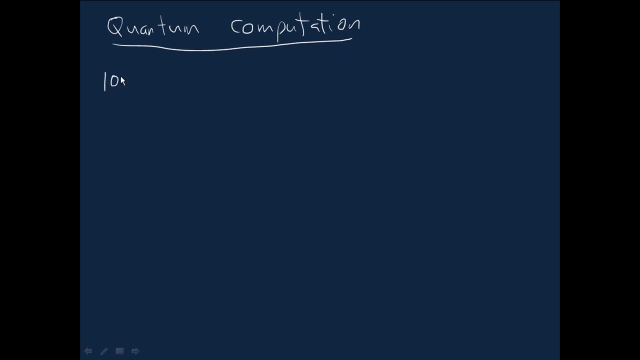 it, and of course it's. it's just a generalization of what we've already been talking about. you start out with many qubits- i'll draw a four here- and then you start applying a quantum gates of various kinds, in particular the single qubit gates and controlled knot gates. 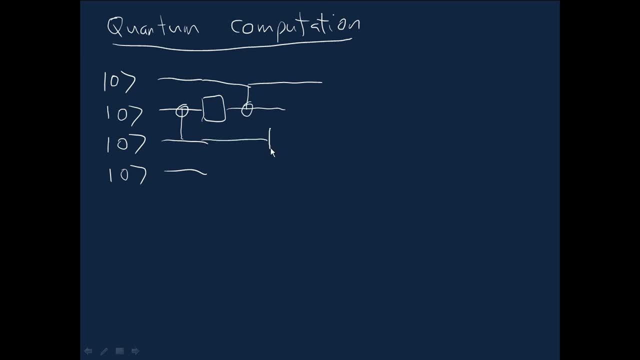 and you can build up an arbitrary quantum computation in this fashion. i haven't labeled the single qubit gates here, but well, you can imagine, you know, maybe some of them are hadamard gates, maybe some of them are rotations, and maybe we've got other gates as well. so that's what a quantum computation looks like at the end. 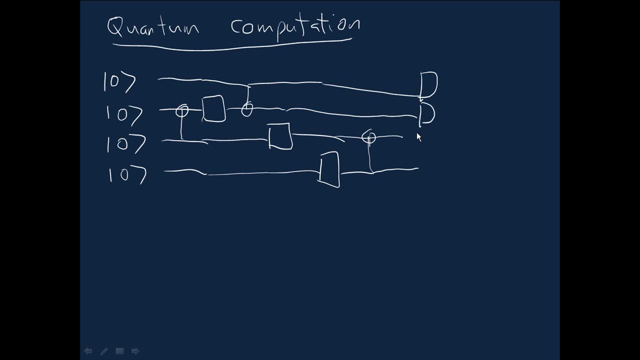 of the circuit. we will typically do a measurement to read out the result and that's a general quantum computation, a couple of little pieces of nomenclature. so i've written here, sort of you know, the zero input state. zero input state, that's just shorthand, of course. 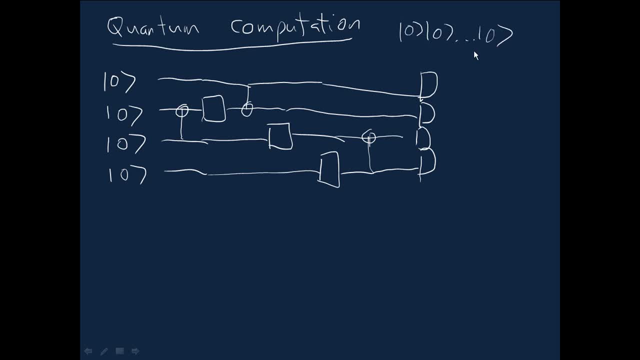 when i write zero, zero et cetera, that's shorthand for the computational basis state: zero, zero, zero, et cetera. okay, so you know. step one: start in a computational basis state. in that this particular case it's the all zero state, but you could start in some other state. 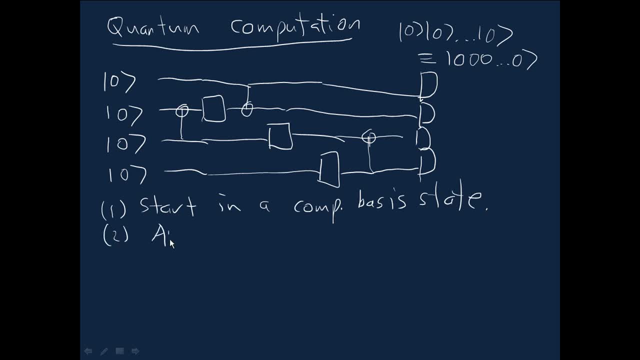 if you wished, and then apply a sequence of uh c knots and uh single qubit, uh unitary gates and that's. that's all uh, uh. quantum computation is except for the final uh, uh readout stage, and that readout stage is just to measure in the computational basis and that gives you your result. 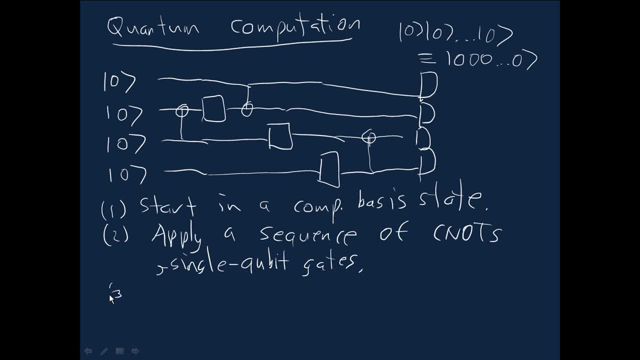 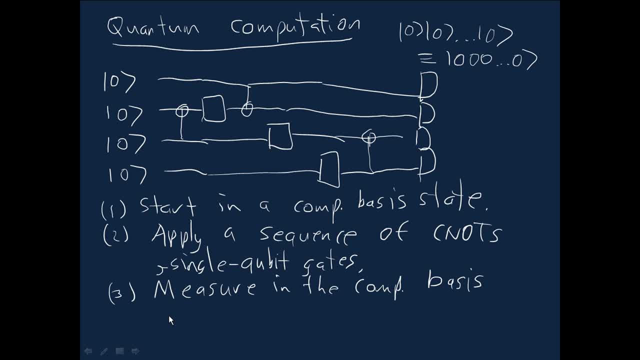 So you know, you get. I don't know something like, for example, the probability of all zeros at the end of the computation is just given by the amplitude you know for the all zero state squared. as you know, as you would expect, given our earlier comments about. 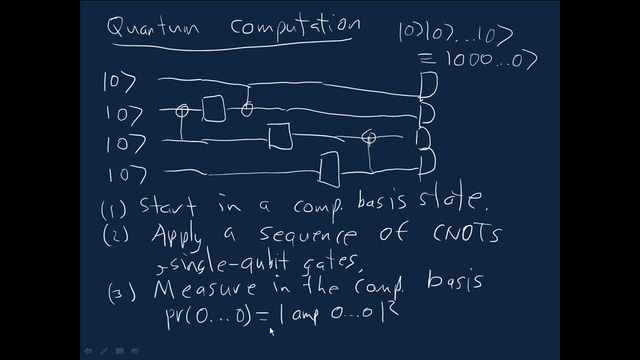 measurement for single qubits. it's the same basic, it's the same rule for an arbitrary number of qubits. So there are some sort of natural questions. you know, this model is obviously inspired by the classical model, but you might wonder, you know what's it got to do? 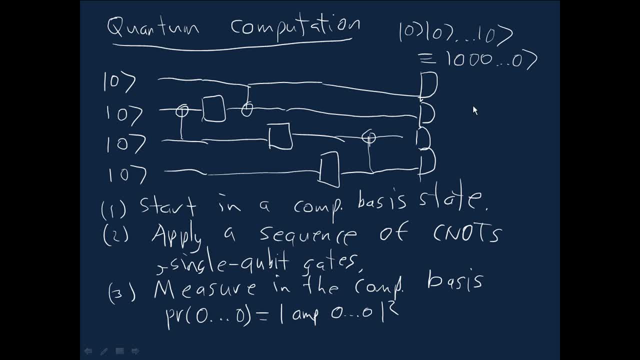 with a classical idea of computation. So the typical classical idea of computation is: you have some input bit, string x, you know, maybe it's a set. you know two numbers. x contains two numbers and you want to, you know, multiply them together. maybe x is a large number and you. 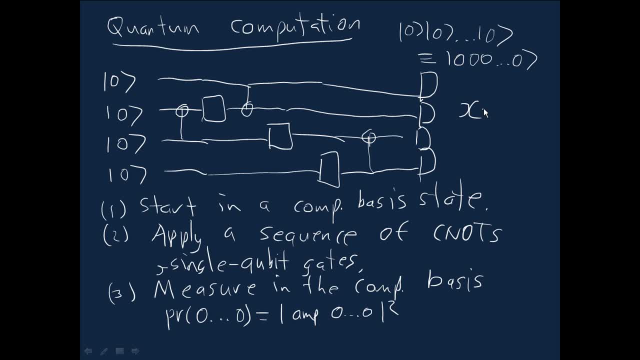 want to factor that in and you want to factor that in and you want to factor that in and maybe you know there could be many things and you want to compute some function f of x, that's sort of the general thing that you want to do in a classical computer And you know. 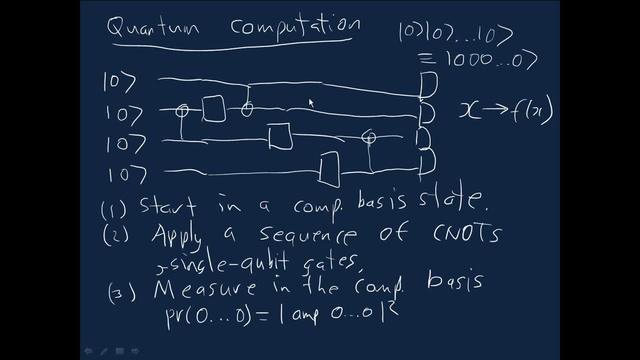 what exactly has this got to do with this quantum computing model? Well, it's simple enough to understand. actually, what you can do is you can imagine that the first you know 10,, 15,, 20, however many bits you know. you can imagine that the first you know 10,, 15,, 20,, however many. 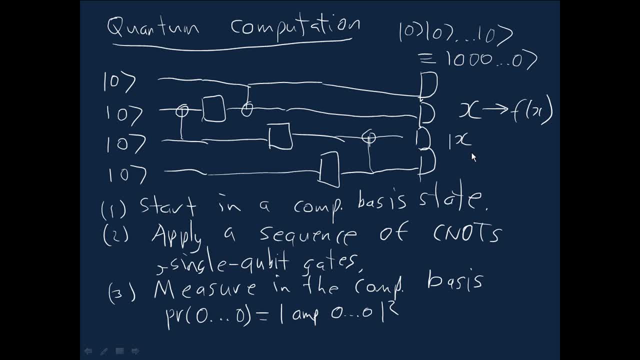 bits store, or qubits, excuse me. store initially the value for x and then there's some more qubits, all initially in the zero state. I'll just write one here, a single bit, and this is the starting state of the computation. so it's a valid computational basis state. and now you'll 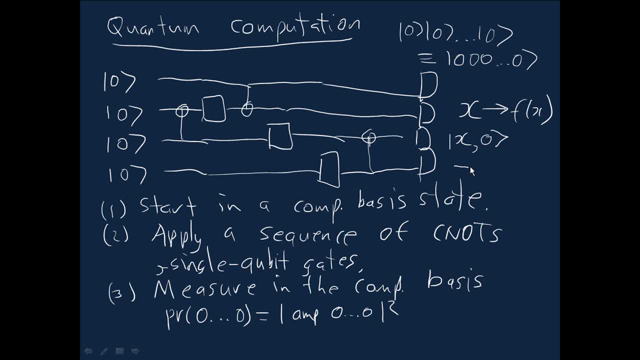 apply a sequence of c-naughts and single qubit gates and with the goal of computing x, f of x. Okay, so you know this. it turns out, and we will actually show later, that whenever you have a classical circuit that can be used to compute this, there is an equivalent quantum circuit of. 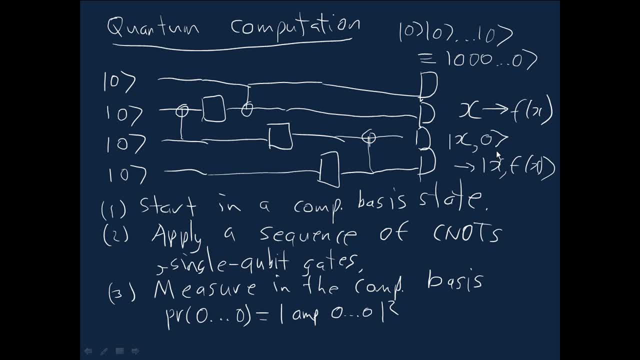 roughly the same size, which computes this down here. So that's the sense in which this contains the classical circuit model. Sometimes, though- and this is the exciting bit, if you're interested in computation- sometimes while there's, you know, it might require a very large classical circuit to compute. 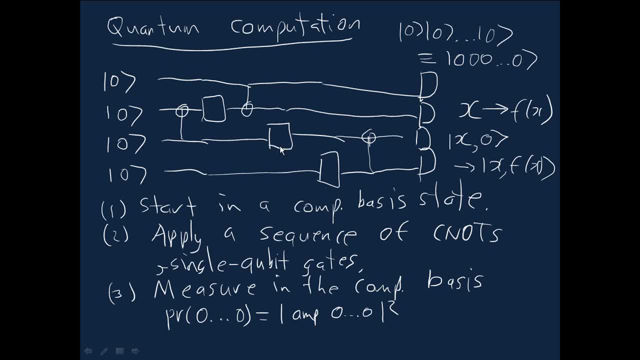 this function. it seems that you can use the greater power of quantum gates, greater power of quantum computation, to actually take a shortcut and to compute this function faster, or some good approximation to it. So in particular, famously, the factoring algorithm of 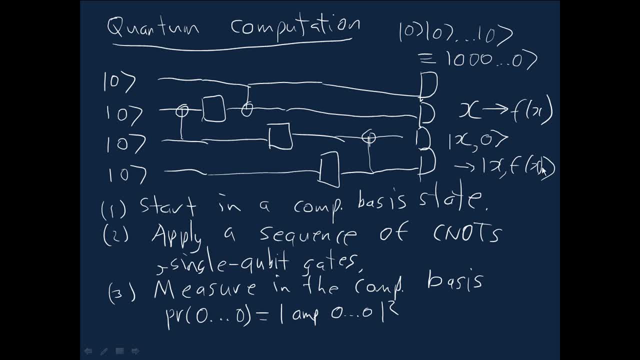 Peter Shaw will let you produce the factors of x rather more quickly than we know how to do classically, In fact vastly more quickly. So this notion of quantum computation can also be used, and we will use it to explain other information processing tasks like superdense coding and 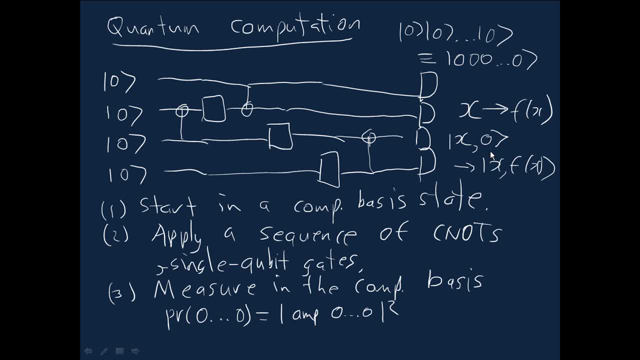 teleportation. Okay, so you know I've described one particular approach to quantum computation, often called the quantum circuit model. There are other approaches which are different to this, some only in rather trivial ways. So you know, it is possible to replace the quantum circuit model with the quantum circuit model. 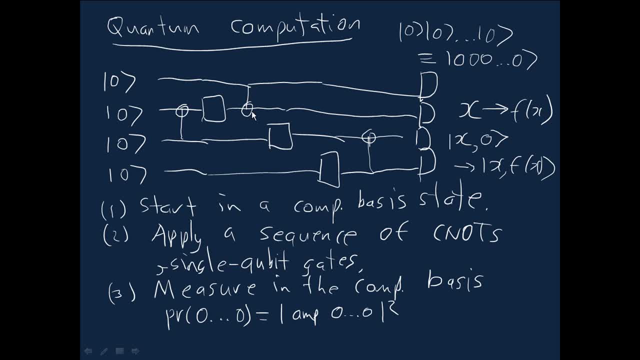 You can replace the control node and single qubit gates by different but equivalent sets of unitary operations or unitary gates. It's also possible to do things like: rather than using qubits, you can use different types of quantum systems, And then there are more exotic models of computation There. 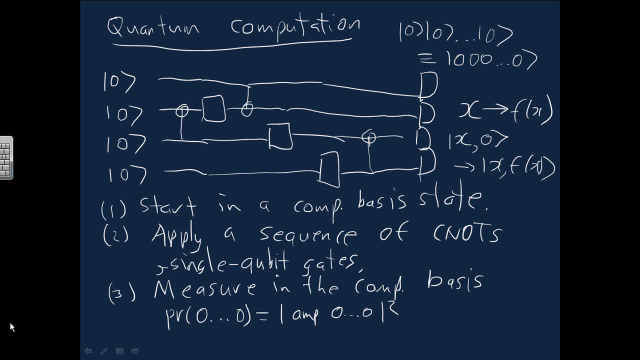 are models which are based solely on measurement, for example so-called measurement-based models of quantum computation, where there are no gates, there are just measurements being done as topological models of quantum computation. And then there are other models of quantum computation where there are no gates, there are just measurements being done as topological models of quantum computation. 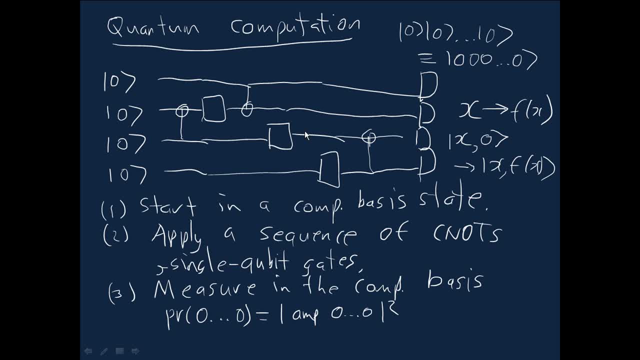 And there are other ones, but the key point for us is that they're all, at the end of the day, mathematically equivalent. Any quantum computation in any of these models has an equivalent in terms of this quantum circuit model of quantum computation. So now that we know in quite some detail, 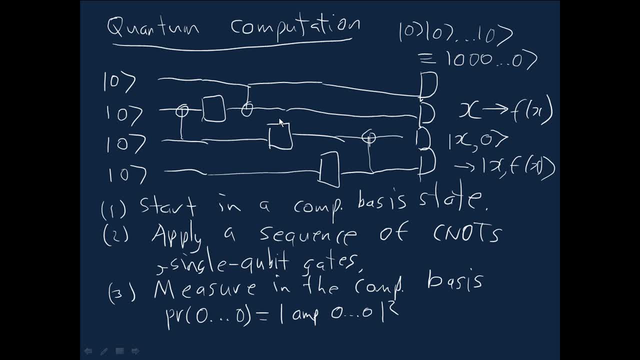 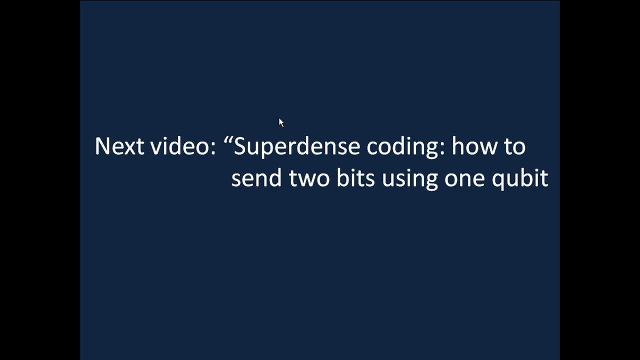 what a quantum computation is. we're going to switch from developing the model to instead exploring the model and understanding what its consequences are. So in the next video, we're going to look at a very interesting information processing task, the so-called superdense coding, which is a way 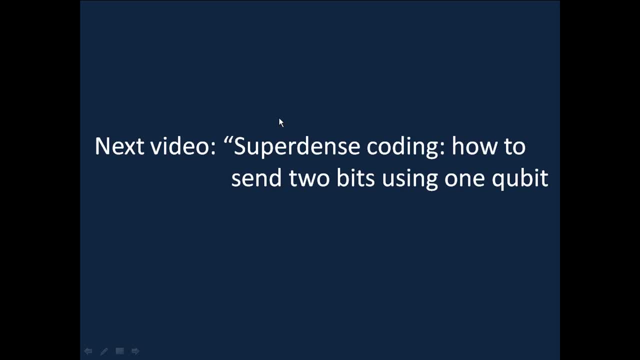 of using a single qubit to in some sense send two classical bits from one party to another. This is both interesting in its own right and surprising. It's also extremely good preparation for understanding quantum teleportation. It's a very similar protocol.